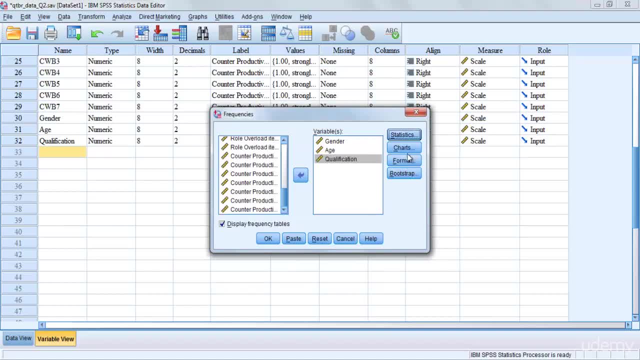 here, but we're not going to select any of them for now. So just simply go on. You can make chart even So. we're just concerned about our frequency table, So we will move on to constructing frequency tables. So let's go to. after selecting, go to okay. So it opens up an output window. You see that? 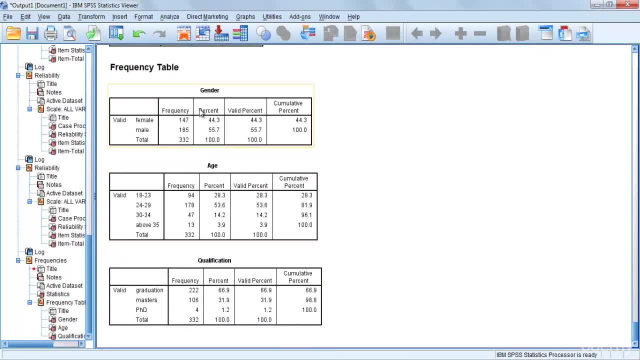 it has given you different options over here and has given you different tables with. it tells you about gender, age and qualification. So there were a total of 32 respondents, 147 were female, 185 for male. And then age, then from 18 to 23,. there were 94 respondents. So belong to this age, then 178 belong to. 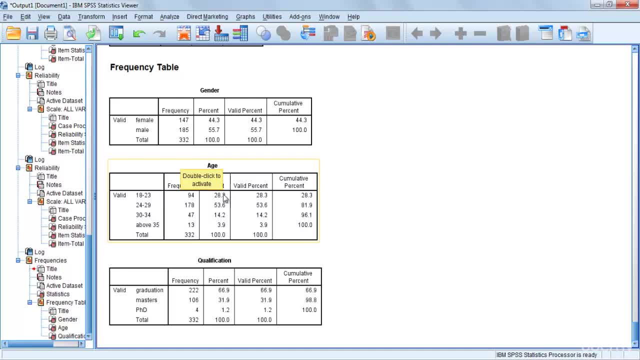 24,, 29.. And similarly, 13 belong to about 35.. These are actually percentages that are of 100%. Then graduation, then Masters, PhD. These are just the frequencies and these are their percentages. Like there's 100%. So what actually you're going to do, how you're? 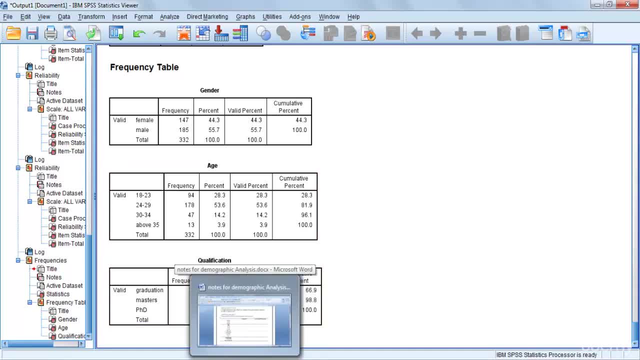 going to perform it. So let's take a look. Protests: Here is how to check. Okay, Now, from the from this grid format, normally I will discuss how to achieve this target percentage. take a look. okay, here now you see that, after performing it, now how you're going to interpret. 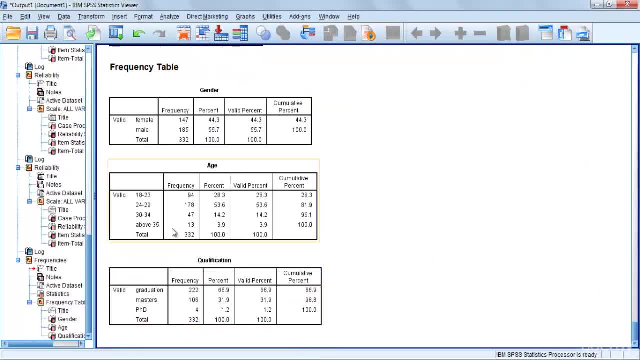 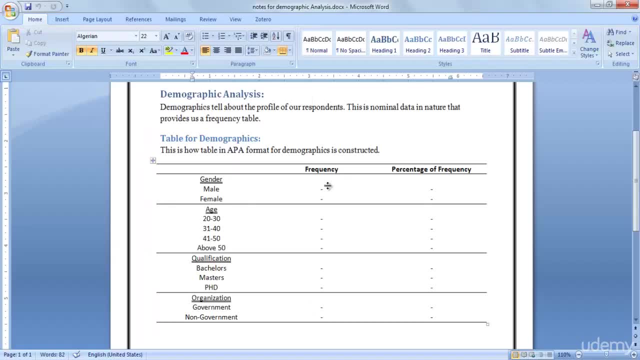 it. this is a frequency table. go back now see here for male and female we're going to write. let's take for male, for example: there were 185 male and then female, 147 female, and then the percentage of frequency. let's take a look. okay, go back to output and you see that there were 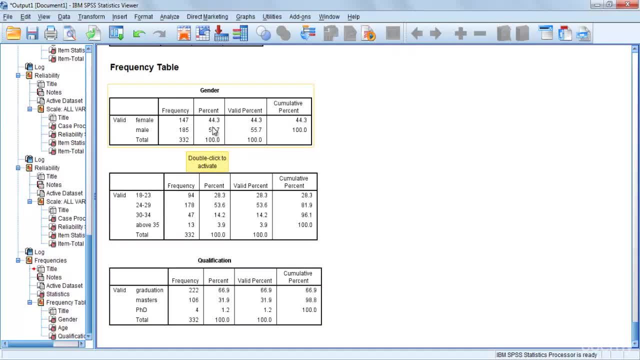 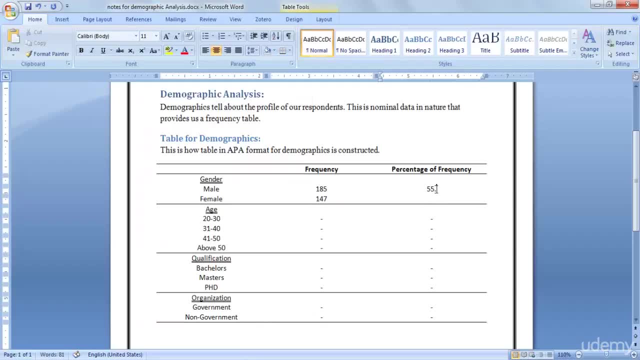 forty four point three female, and there were fifty five point seven mean. so just put it in your table: fifty five point seven percent male and then forty four point three percent female. let's you can put percentage sign as well. so this is how you're going to interpret the others as well in the form in the.